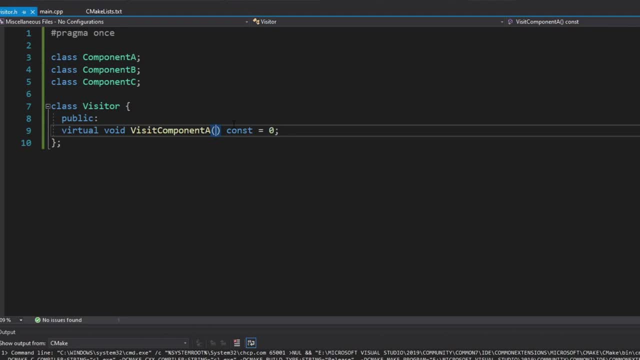 so let's go ahead. and well, we want to pass in the element we're going to operate on here. So we're going to go const component A. and what are we going to? We can call this element or whatever we want to call it. We'll call it com. So we have a visit. 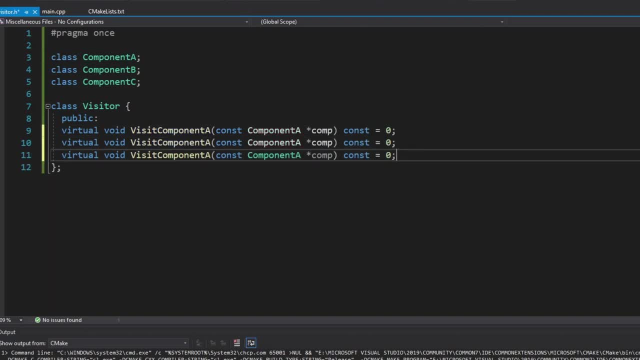 component A takes component A. Okay, kind of weird, right, I don't know. Let's make a couple more of these, though It'll make more sense here shortly. C there, All right, so this is the main interface. then, Obviously, it's pure virtual. You can't instantiate it. So where do we go from here? 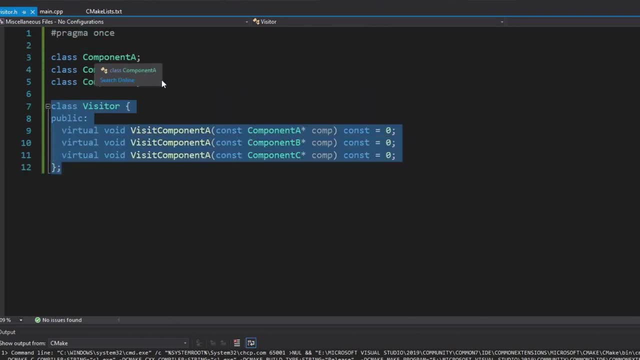 All right, well, we'll get back to that, but these things have to be in a certain order because, just the way the header order is, and it knowing about things, it only knows about things above it. So let's go ahead and do that. So we're going to go to the header order And we're going to go. 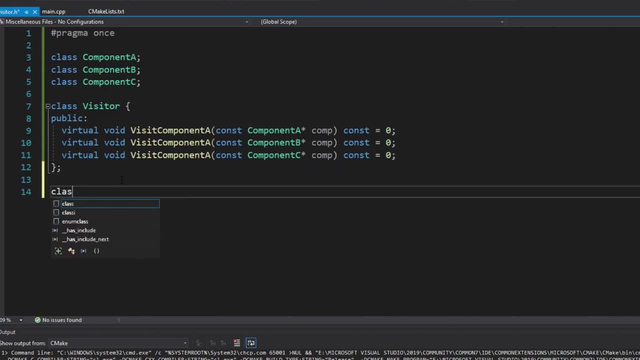 ahead and declare our base component class. So this base component class, we want to also make an interface. So this one is basically going to have. let's make a destructor here And there we go. That's just wired. You might actually want one of those on the visitor too, but we're going to. 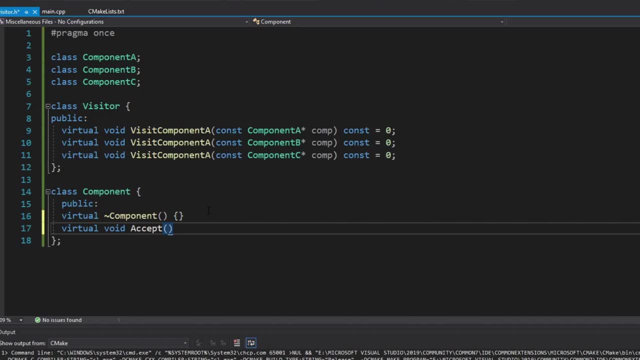 skip it. And then we also want to have an accept. So this is going to accept a visitor and we want to do it as a pointer. Naturally it has to be a pointer, because this is a pure virtual class, So it can't accept a real instantiation of that. It has to be like that And that's all we need. 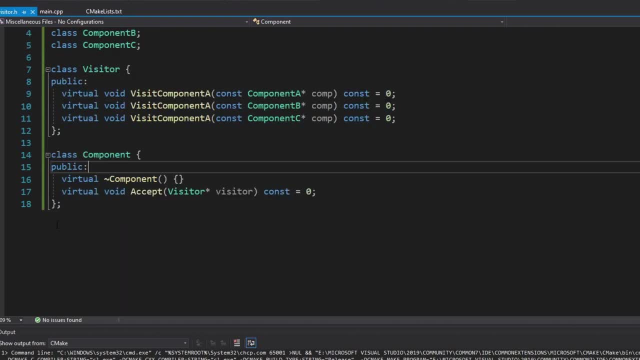 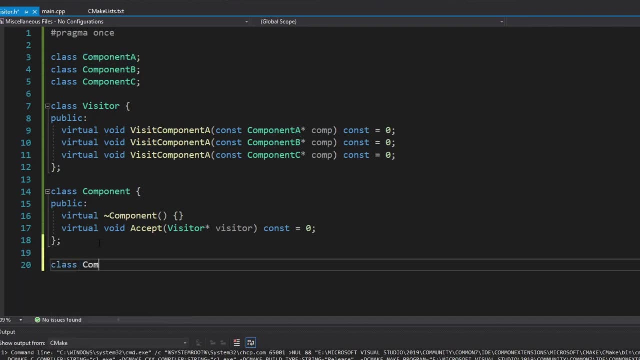 for the component. So we got a couple of interfaces here in that order. So now what we want to do is just define what these actual components are, So we can just go class component day and that's going to be public component And we're going to have a public method and we got to make this. 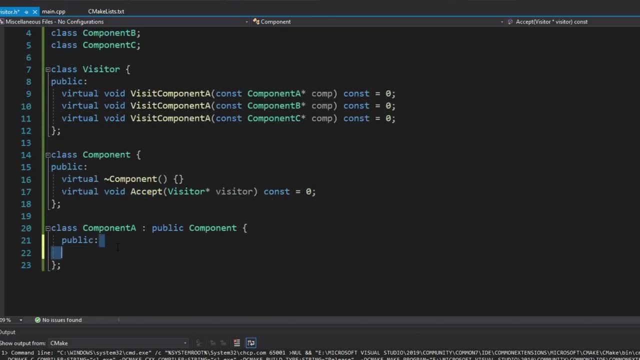 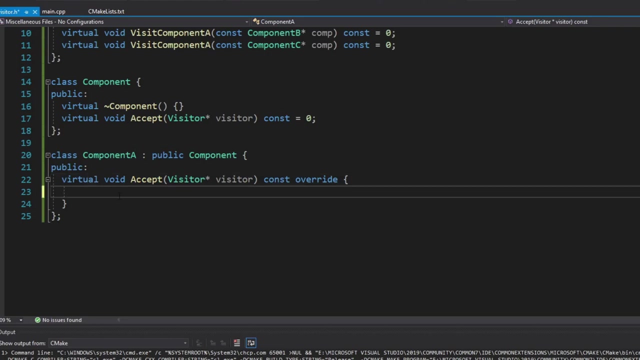 accept method here work. So we at least got to have that. So we just go virtual void, except visitor, star, visitor, same thing, const, and then override And what's going on here with the formatting. there we go much better And basically we want to have this one. 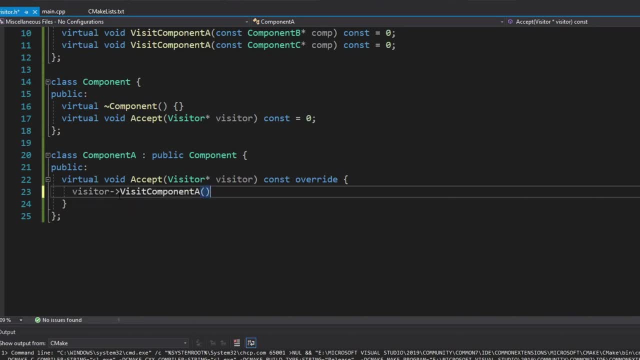 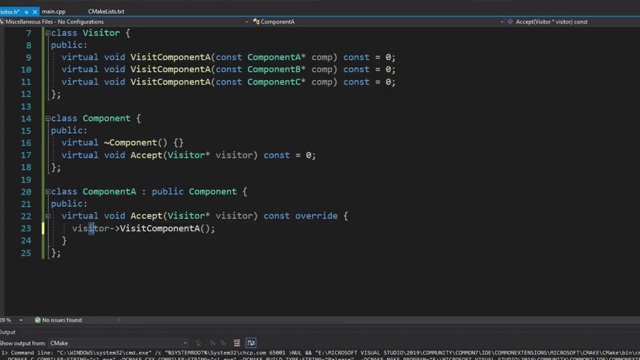 call what you would expect: visit component A. So there we go. Now you can see how that would work. if you instantiate component A, If you pass it some kind of visitor, it will call this visit component A, function which they must instantiate. But the important thing here, 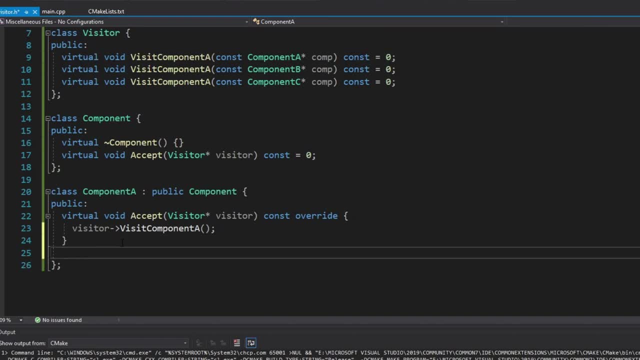 well, interesting thing here is all right. so these, any of these public functions the visitor can do stuff with. So you want to have some public functions here to do stuff? Let's just- I don't know. we'll return some strings- Say, maybe you know, maybe you have a get name or 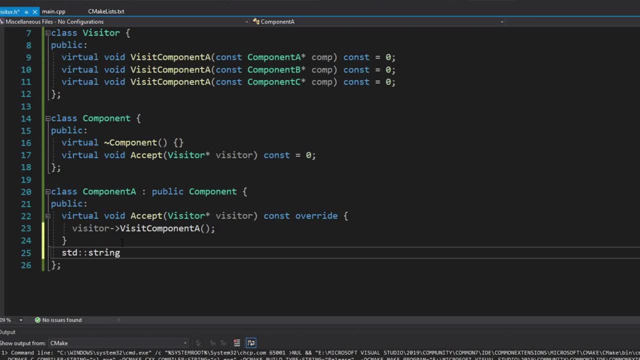 get something about it and return the string. That could be. that could be fine. So we just want to go like component, A function, I guess. Sure, We don't necessarily want these all to be the same name, That would get confusing, but we just want to return. oh no, we'll just return. 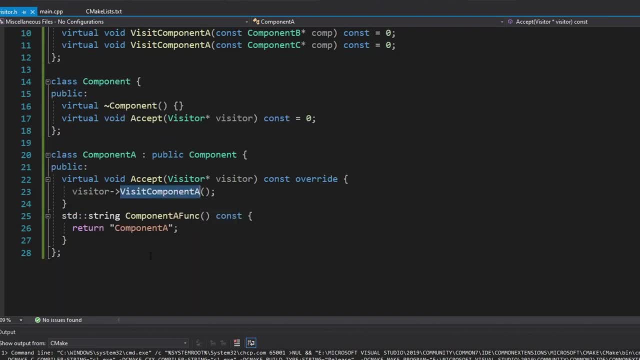 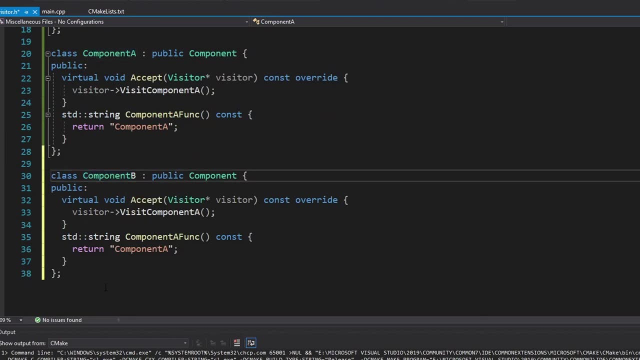 component A, So that visitor takes care of that, All right. So let's make a couple more of these. Let's make component B, component C. you know you want to make as many as you need and or whatever you need. So we'll just change all these to B and let's do the C as well and overkill. 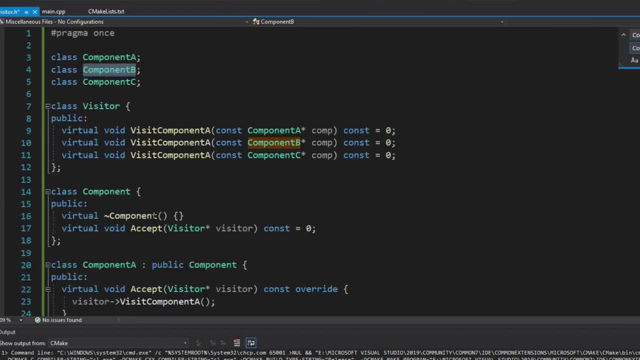 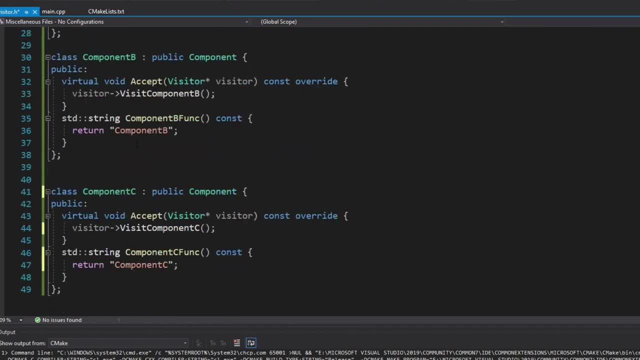 at this point, But this time we're just going to use a quick find and replace. We got to make sure we get these functions right. Yeah, Make sure we're calling the right visit, Okay. So we've got all that. Now we just need some visitors that implement these functions And, as you might imagine, we're 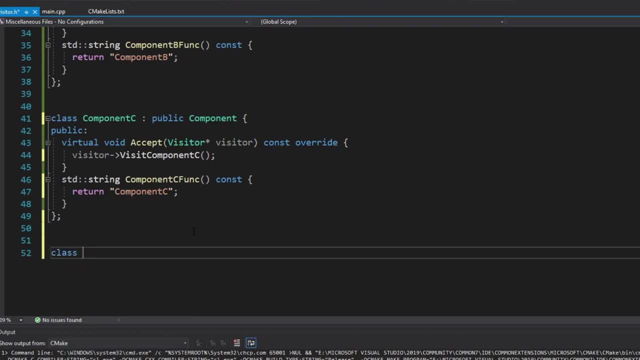 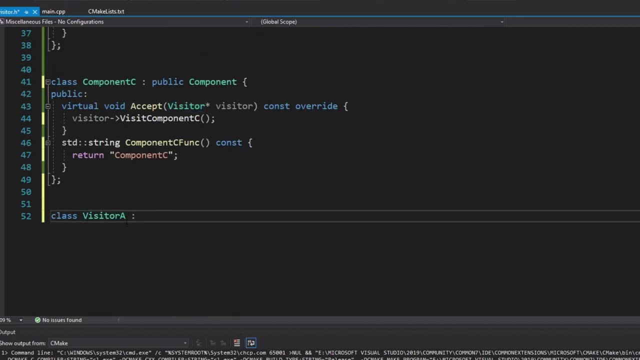 going to make a class For each one. So we're going to make, let's see, virtual ones called visitor. Other ones don't really have a name, I don't know. We'll just call it visitor A. These are the real ones. 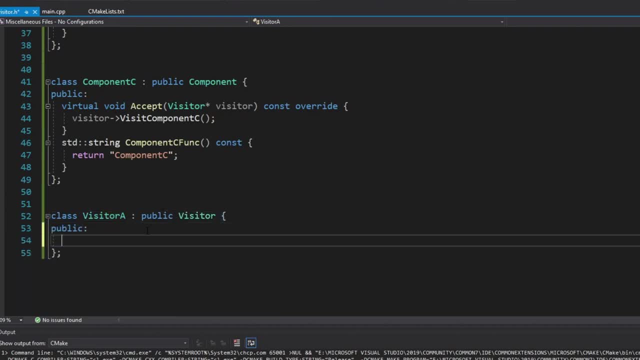 ones you can actually instantiate And basically we would just want to have some special functionality for any of these. Actually, I don't want to call these A, B and C, because these visitors could be applied to any of the components. They just they basically want to do special. 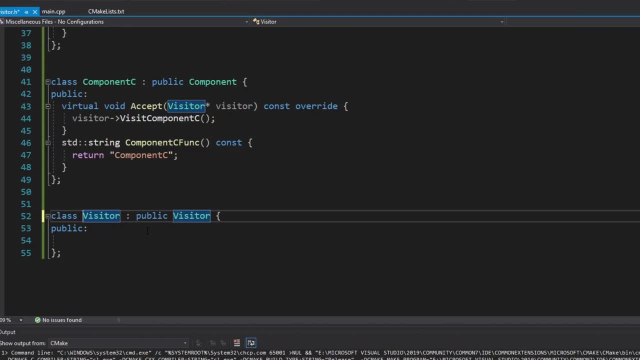 functionality based on what this visitor is for. So maybe we'd have like a trying to think of something. I don't know, You're going to have to use your imagination. I'm not really coming up with anything, but essentially these would do different. They would do different things as they visit and have some 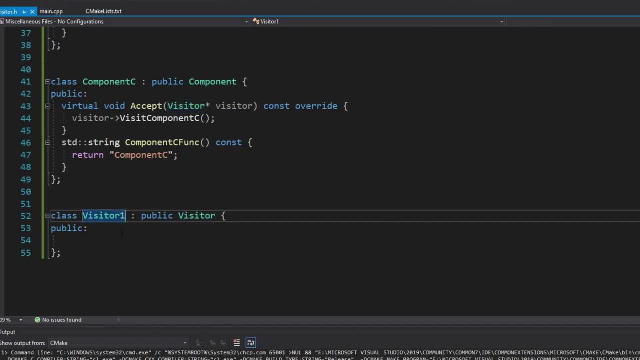 special functionality. I guess for now I'm just going to give them numbers, Yeah, Instead of letters. That way they're not you can. they're not naturally associated by lettering because people might think, oh, A only works with A. That's not the case They all. interchange would be the. 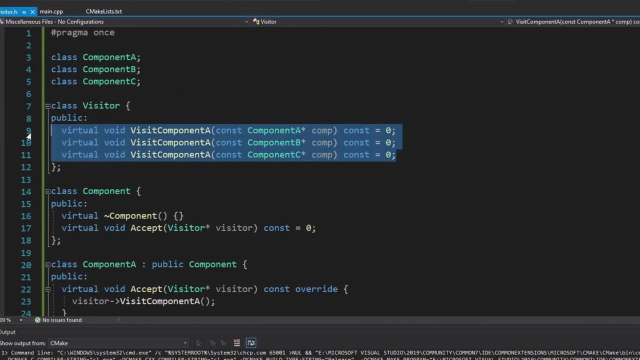 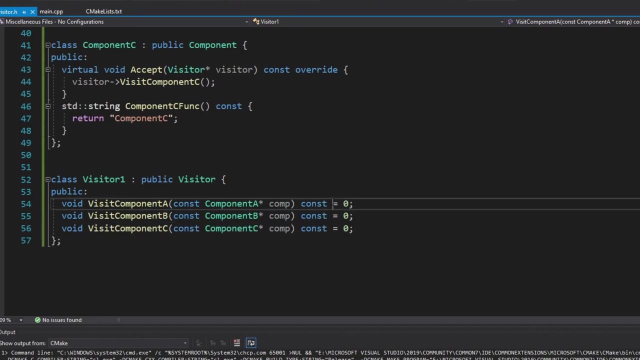 point. So now we just got to implement all these functions here and determine what we're doing with them. We're going to call these with: oh, hold on, We made a little error here. Got to actually give these different names: A, B, C. There we go, Okay, So now the visitor can either visit A, B or C, and we need 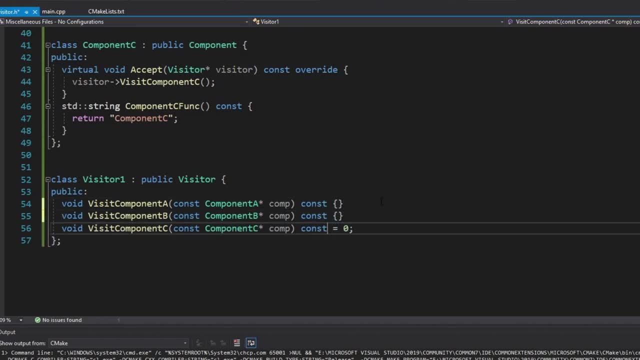 to give it some kind of function definition. We might just return for now, but now let's do a quick CL. All right, let's make them log, and we're not using IO stream at all until we get to here, So I'm 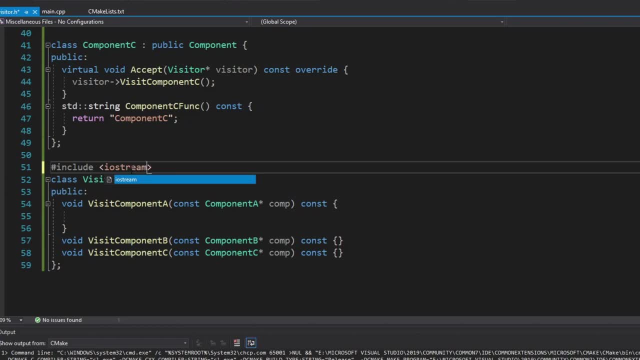 actually going to put the include IO stream right here, which I know seems awkward, but sometimes when you're doing header only stuff, this is how you want to do it. It's just kind of a fact of the header only method here, because this is all getting built into the 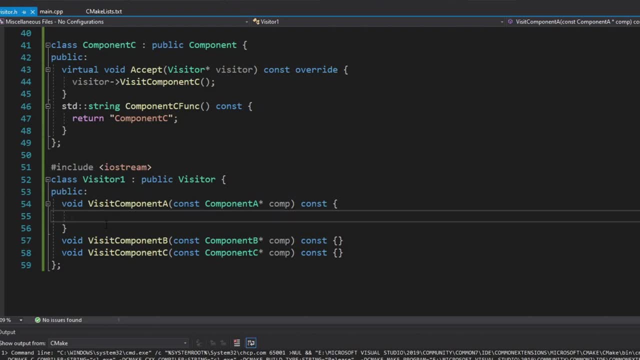 main. So you want to you care about the order of things a lot more when you're doing it like this, but disregard that overall, because that's kind of a side point just about the way I'm doing this. All right, So let's use C out here And basically we want to go well. 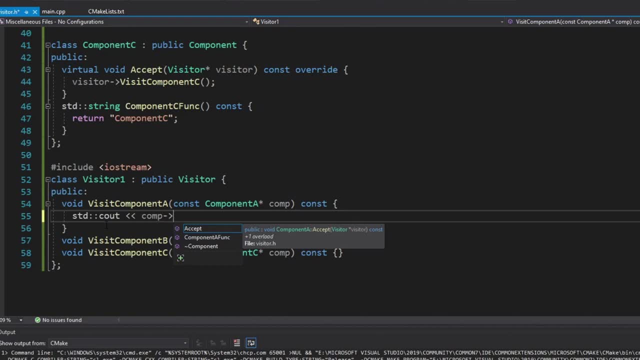 we'd say this variable comp, and then we call its method. except we're going to call specifically component A method here. So that's the one we're passed in, That's the one we have access to, And then we can say: well, we'll put like a visited here, Let's go visited. And then it'll say: 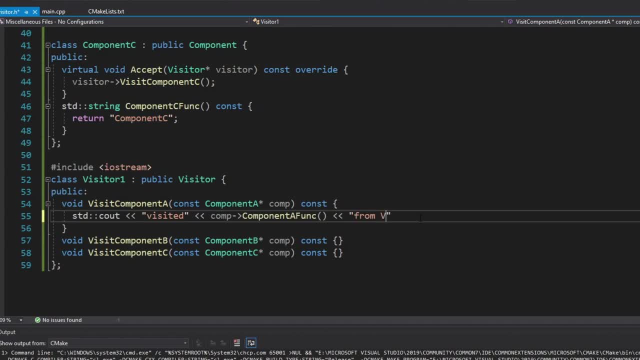 whatever one of this, and then we can say from a visitor, one Cool. And we can basically do the same thing for all of these, except propagate it down, Call the right function, And this will be B and this will be C, So you can make as many visitors to do as many special things as you want. 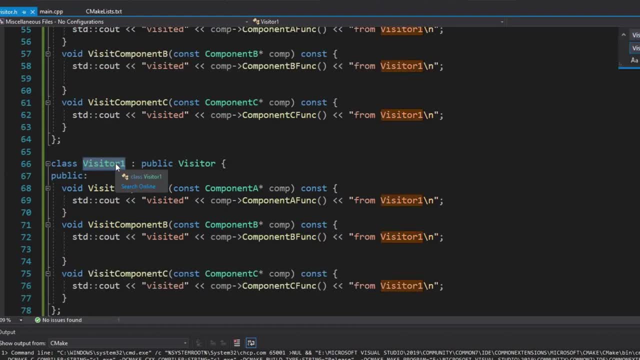 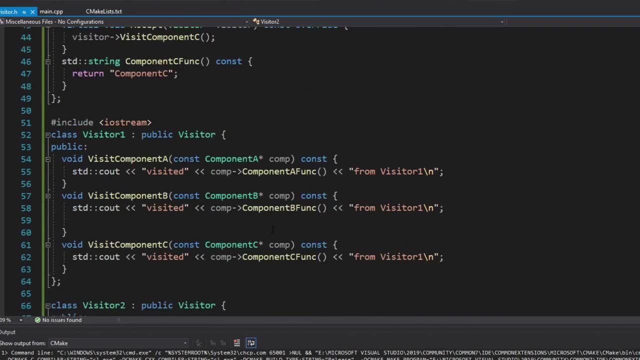 For example, we'll make a second one- Let's call this visit or two, and we'll do some replacing and go. Visitor two looks good, Visitor one looks good, And you can imagine we could add a third if we wanted, and it'd be, it'd be fine. But now let's go back over to our client code and run. 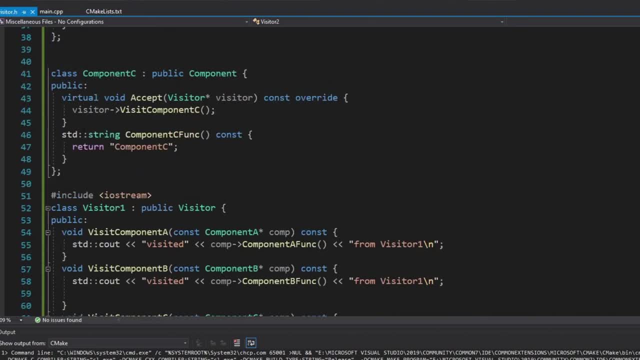 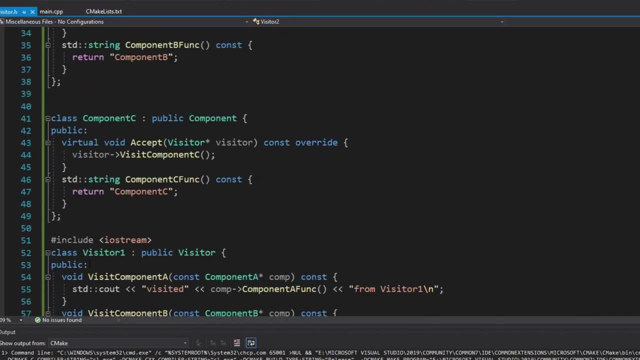 include visitor. So we can start working up an example And typically when you're doing this you may have like a big array of things And you'll see kind of the point is, as we add functionality with visitors, we don't have to edit the components anymore. The only thing we had to. 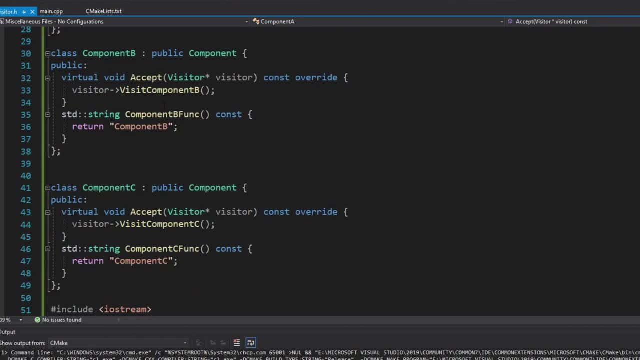 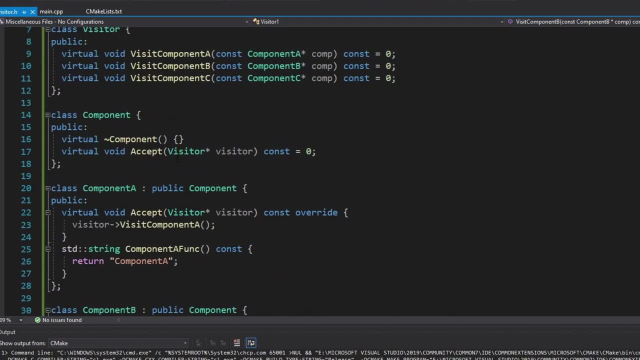 do was just one time put this accept method in, and then we can have all kinds of different visitors that do special things publicly, And if you want them to have private access in any of these, you have to do some kind of friend thing. That's a whole nother avenue. All right, let's, let's do. 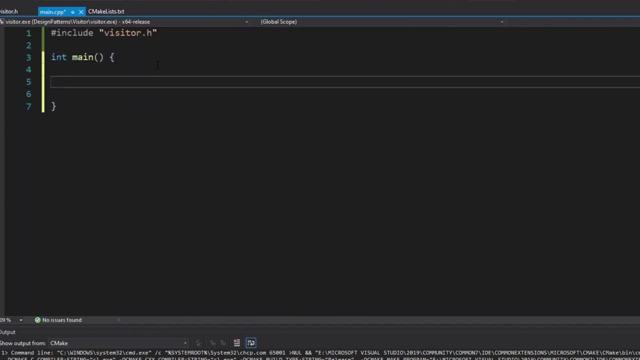 some examples. All right, let's go over to our main And let's let's see how we're going to do this. I guess we could use just like a vector or an array. Let's do an array. I'm gonna go off. 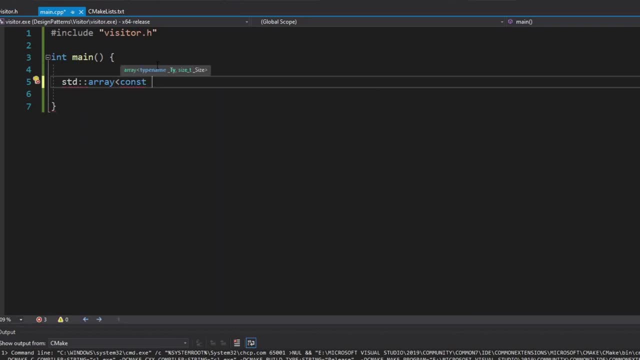 another example. I saw that I kind of like this vector. it's going to be an array of what components. it's going to be An array of components. Oh, I copied everything And we can say components. Now, what's this confused about? I don't think it knows what array is. I think we got to include array here, Yeah. 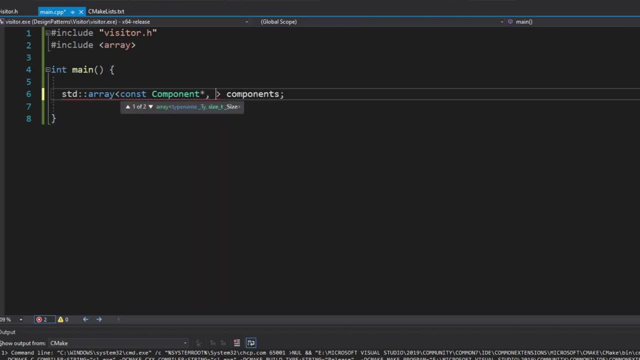 that's it All. right now, it should be a little happier. This was an array. we also have to declare how many. let's just say. let's just say three. there we go, And now we're using the array syntax correctly. So three component pointers. this is essentially the same as doing it the old 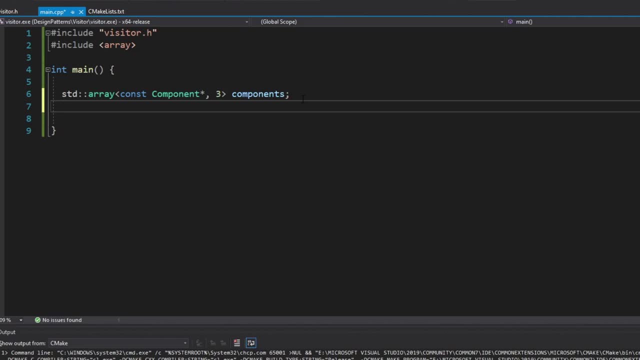 way of making arrays. But just yeah, that's fine, So let's instantiate these. I guess we could use instantiation via this method: new component a, new component B, new component C. I'll use this syntax too often because it always. 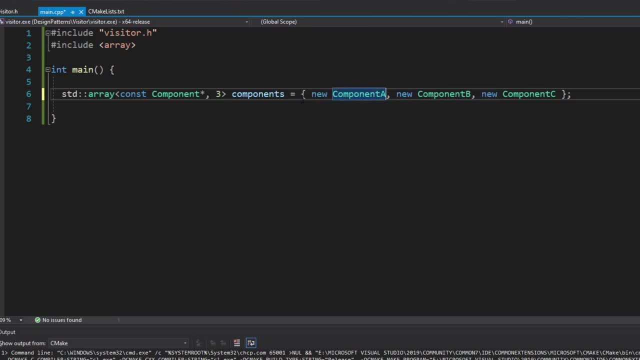 feels awkward to me, But we'll go ahead and do it. I always want to do something like: don't you gonna try to do this? Well, you can do it either way, Either is fine. It understands what you mean. Okay, so we've got three components. 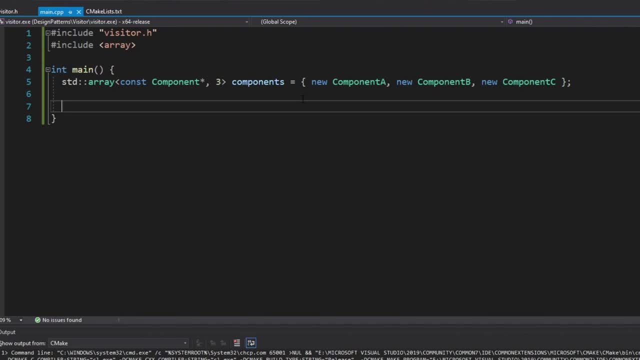 And now we need some, some visitors. So let's make some visitors. So let's make visitor one And let's make visitor two as v2.. I don't necessarily need to make them first, But those are the ones we have, So we're. 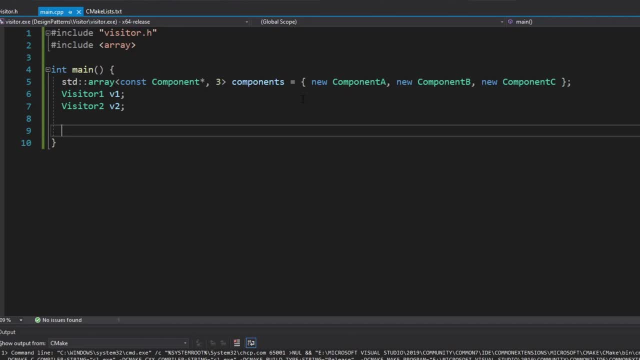 making them quickly. And now what we can do is we can go over all these components and run either visitor on that, So you might have a function for this that takes in this array specifically by reference or something. But you could also just go and just write to the for loop and just say: 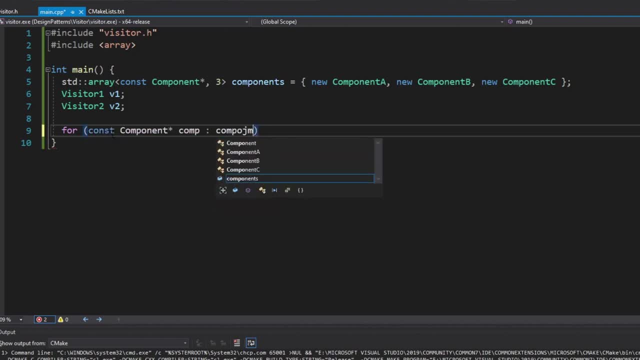 const component and components. Spell this right, there we go, And then you might run something like: well, we just want to call, except all of them, And we want to call it on, let's say, v1 the first time. Now, what's wrong with this? Why doesn't it like this? Let's have a quick look. 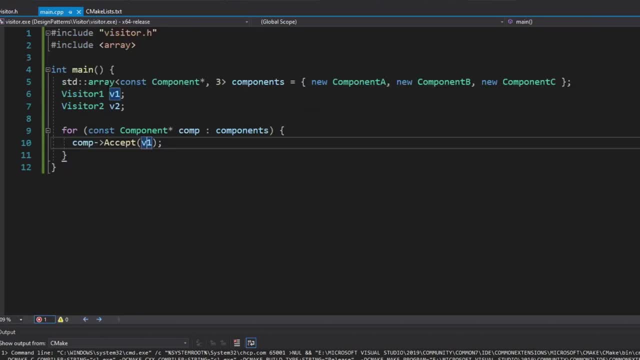 at visitor. We're at our component. we want a pointer, All right, no problem. So we could do this two ways. We could either sleep through it like this: we can just make these pointers- There's also ways to. you know, we could put a reference symbol on there and it would figure out. 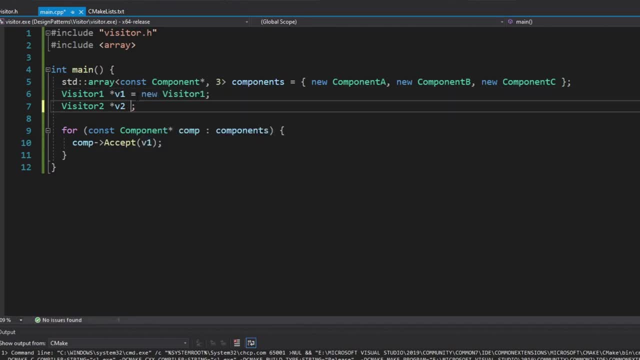 too. But let's do this: There we go. Now it just knows what they are. So we can do that first, And then we can go, and we can do it again, this time putting visitor two on it, And let's just go ahead. 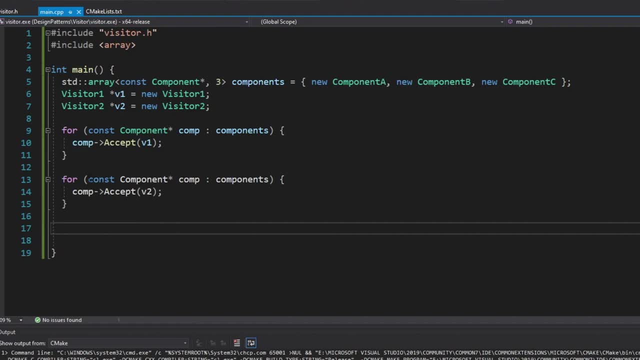 and see what that looks like. So I'm going to switch this over to visitor. make sure C makes ready to go. It looks like it is our. let's just hit play. We got a warning. Let's check out what we got. Looks like it just doesn't understand what a string is, So let's go over to visitor. 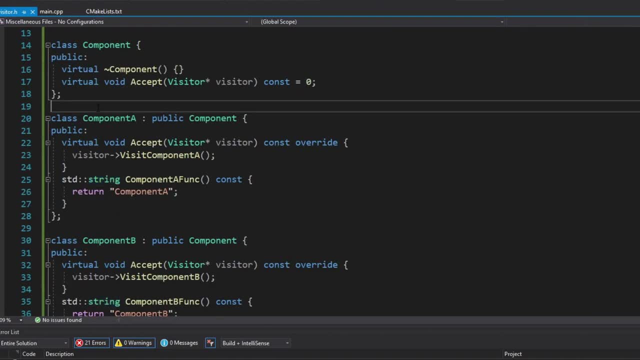 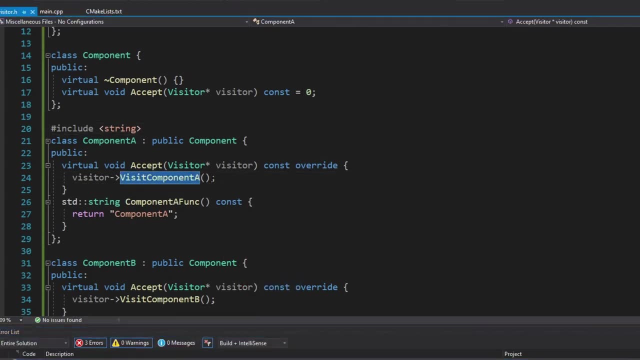 and find where we first use string. It looks like it's on these components, So let's just include string before that And hit play again. must have one more error somewhere here says component A does not take zero. Oh yes, we have to pass it, the class. 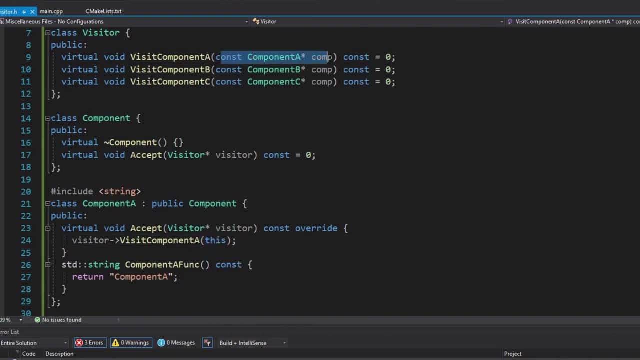 So you do that with this keyword. it wants a const pointer to the class of the component. And well, we've got the class where inside of it, we just need a const pointer. And this is a const pointer, So we need to put that in all of them and then hit play. 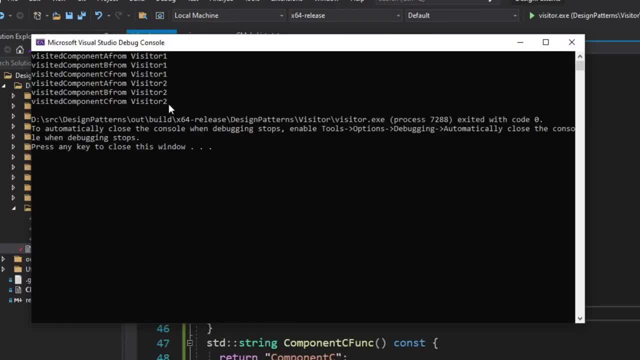 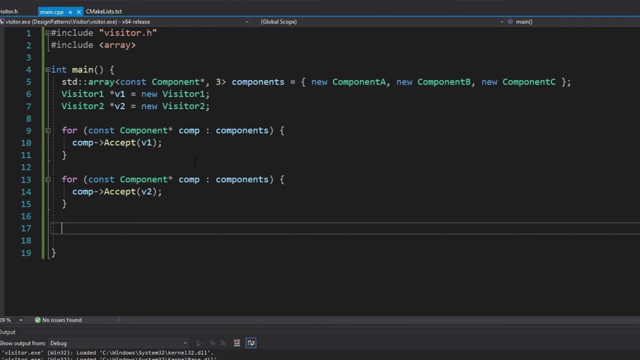 And there we go. we can see we visited A, B and C from one and two And that's essentially the whole pattern And of course we want to clean this up and delete all the stuff. So we'd probably do this one more time and say delete, comp, delete, and we are exiting the program. 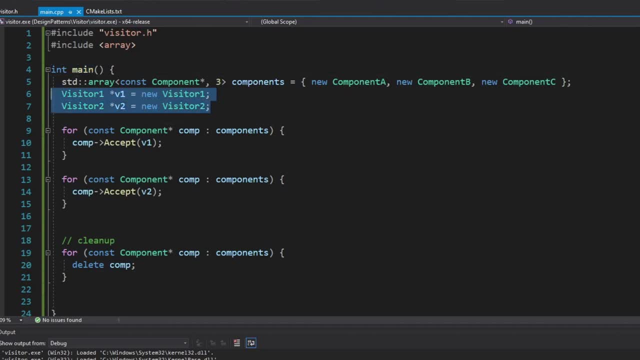 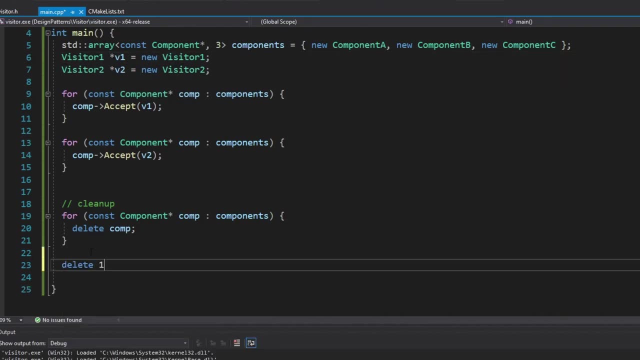 So this doesn't actually matter, because it's going to clear at the end of main. But if you're deep inside your program somewhere, it doesn't necessarily clear. we can also do the same one same for these, But it's good practice to do such a thing And we return zero, All right. 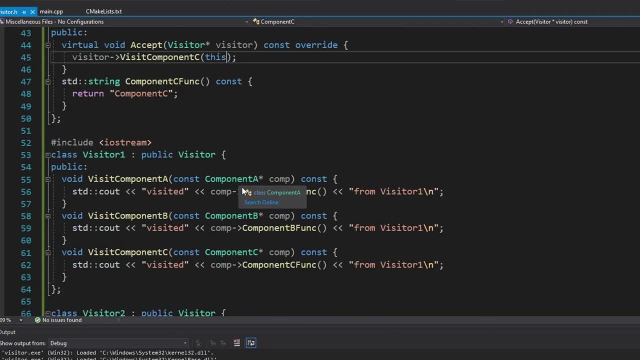 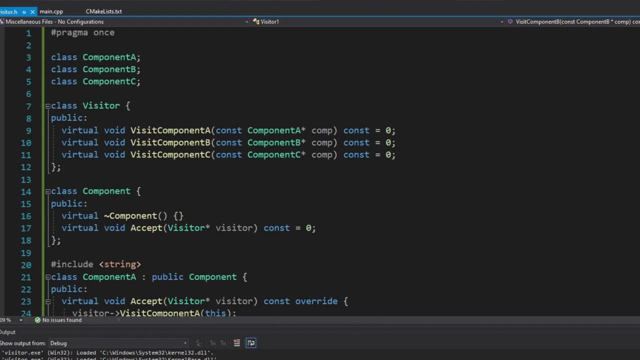 I think that's pretty much it. I don't think there's a whole lot else to it. Just study that example carefully. It's it's going to be the same in general always with the visitor. there might be a few different hacky ways of doing it. I was kind of playing around.